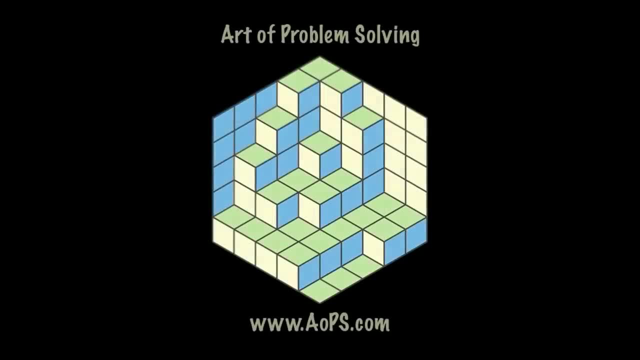 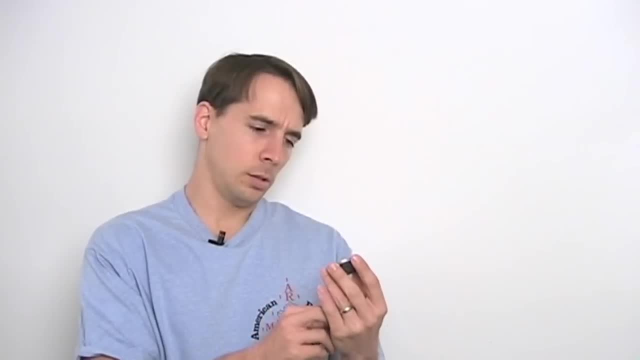 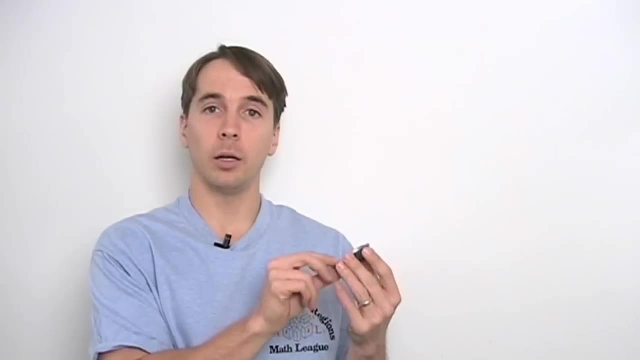 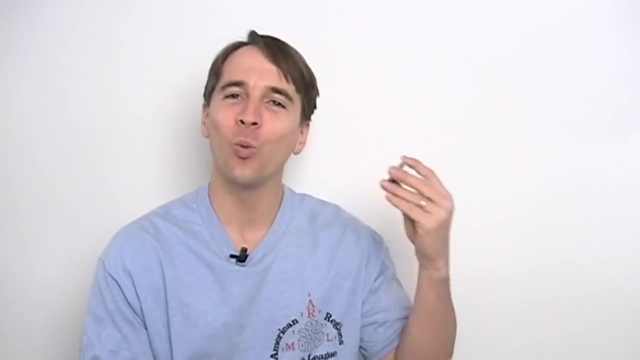 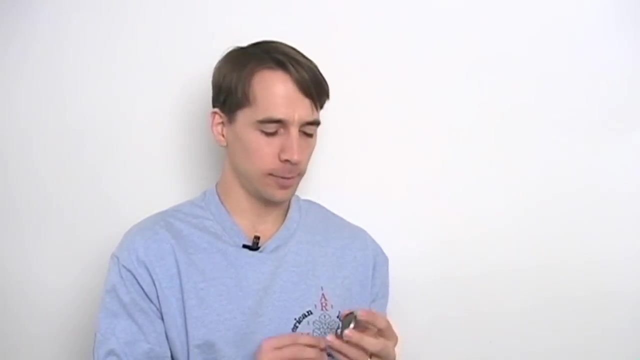 Look at this medal I found. On the front it says United States of America- Mathematical Olympiad And on the back it says Richard Rusick. There's only one of these in the whole world. Very special, very special. There's only one of these in the whole world because I was only a winner of the Olympiad once. 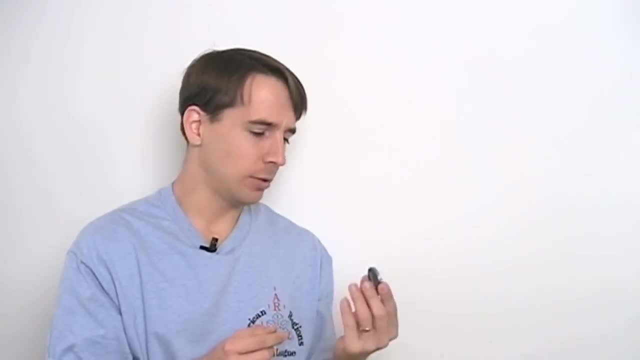 But it is still a very special medal. I mean, well, it's not that special, I haven't really used it for anything, But I'm going to get to use it today, because we're going to play a game with this medal. 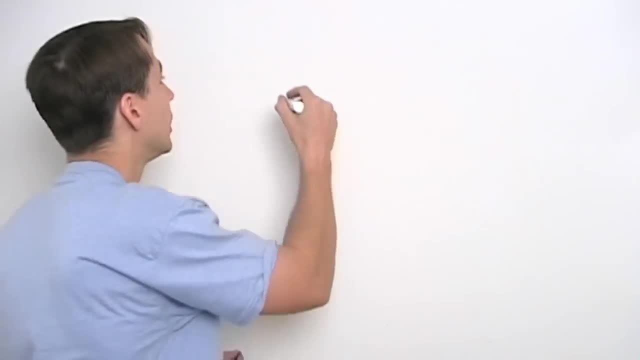 And I know how much you like games. What we're going to do is we're going to start with a number on the board- Number on the board- And the number we'll start with is 1.. Well, we start with 1.. 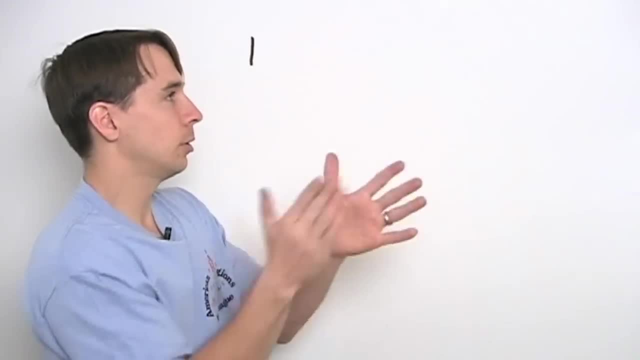 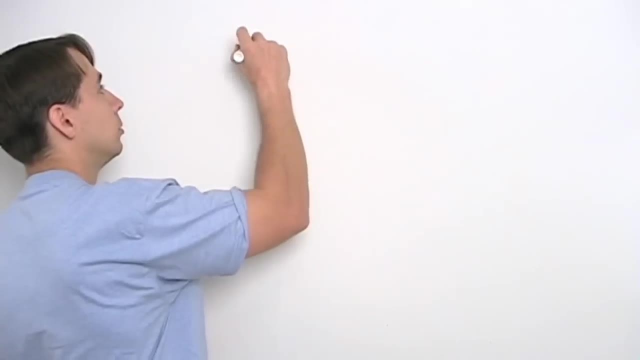 And we're going to flip the coin. And we flip the coin And it comes up with the Richard side. If it comes up with the Richard side, what we do is we double the number on the board. So you like it. You got a root for me here, You like it. 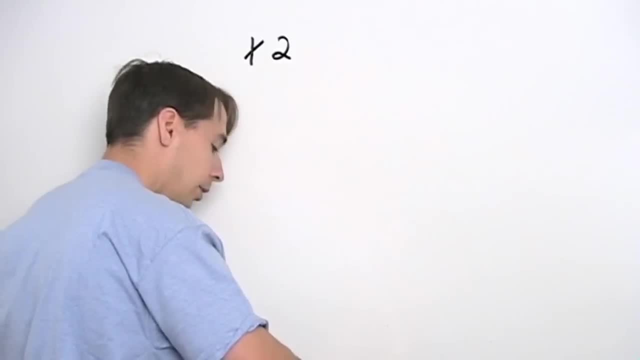 When the Richard side comes up, because we double the number on the board, And the reason you want to double the number on the board is at the end of the game you're going to get the number of dollars that's shown on the board here. 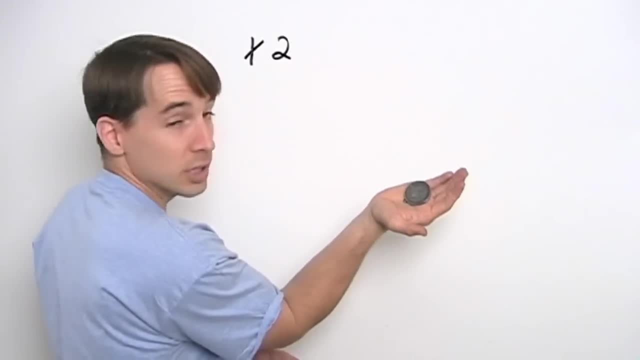 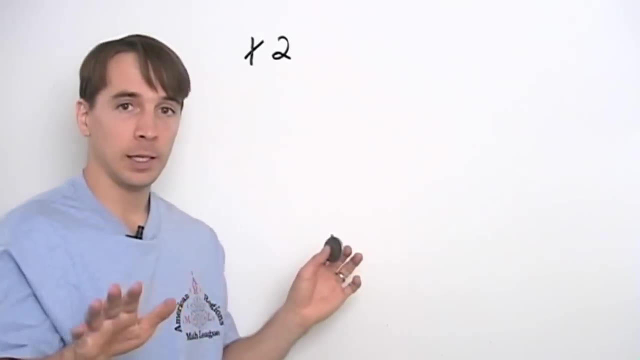 Now, how does the game end? Well, what if we flip and we come up with the USA Math Olympiad side? That's how the game ends. We flip, It comes up with the USA Math Olympiad side. Game is over. You get the number of dollars that's on the board. 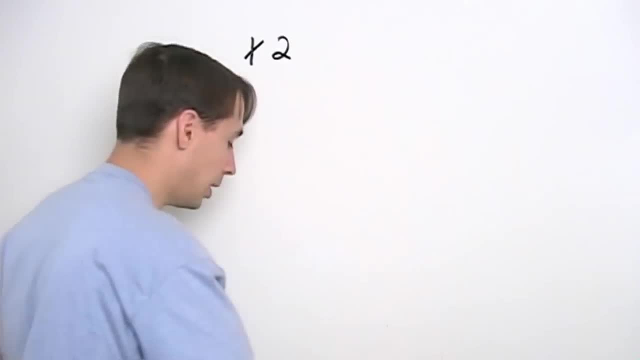 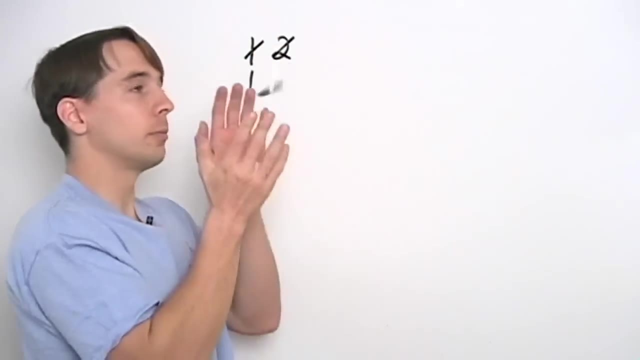 All right, You got the game. We're going to play it a few times here just to make sure you got it down. So we'll cross this off And we'll start with 1.. We always start with 1. And then we flip, We flip. 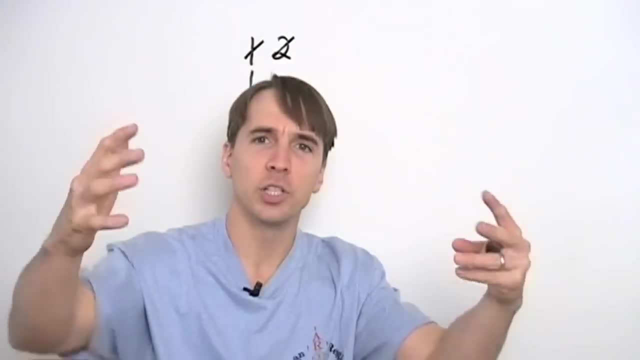 The Richard side. That's good for you. See, you got to be rooting for me. You got to say go Richard, Go Richard, Let's hear it, Go Richard. You're not rooting for me at all. Not rooting for me at all. 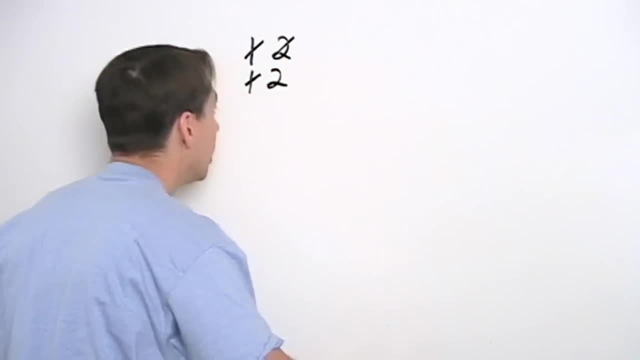 Not rooting for me at all because, well, you've seen the other games I've played And you know there's a catch. You know there's a catch. Let's see. I'm going to keep playing, Then we'll see the catch. 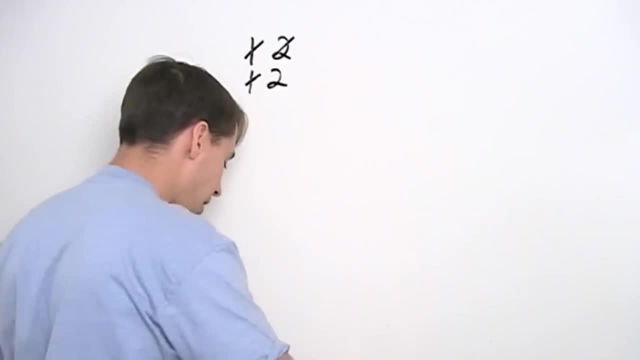 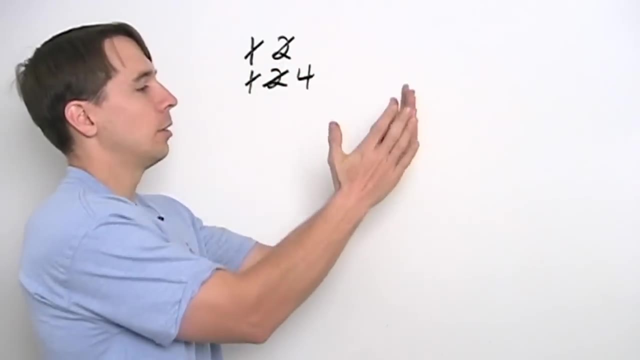 All right, Flip again. Richard Got the Richard side again, So we're going to double that up And that is 4.. Oh, we got the USA Math Olympiad side, So we stop And you get the 4 dollars. 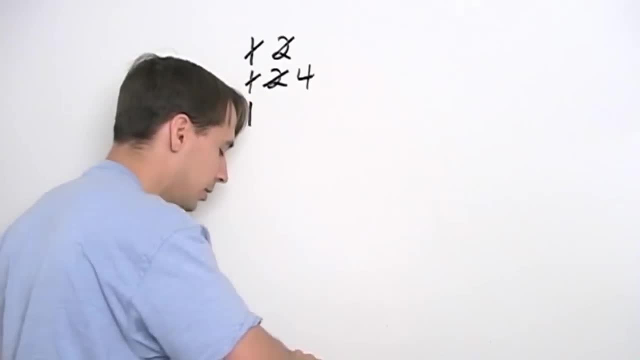 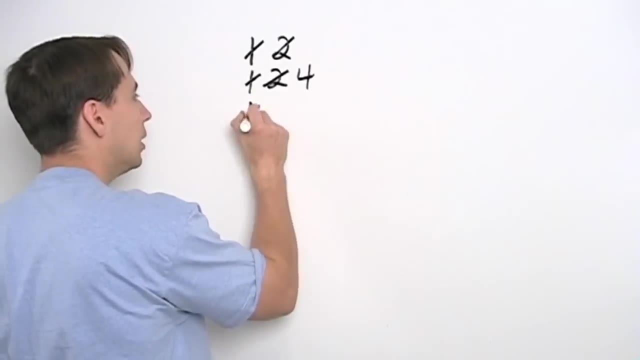 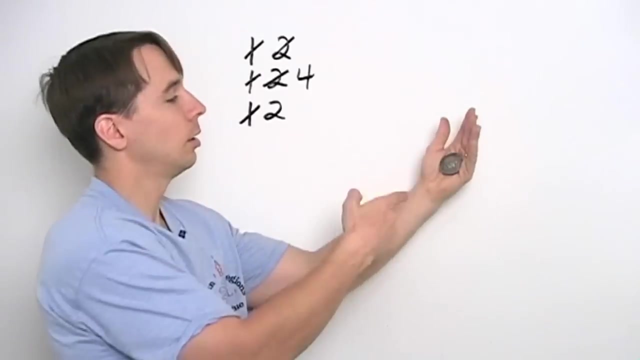 We'll play again, Just to make sure you've got it down. Start with 1. And we flip. Oh, you got the Richard side right off the bat again, So you double right away Again. Cheer for me. I want to hear it All right. 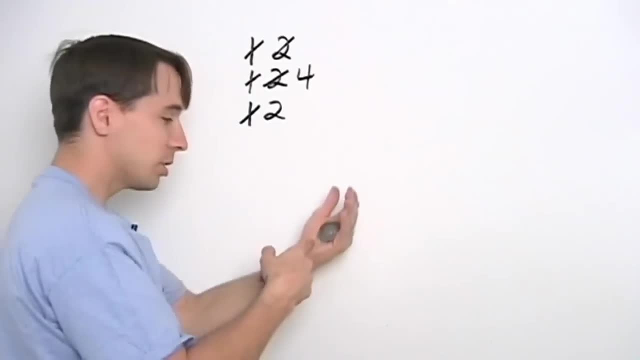 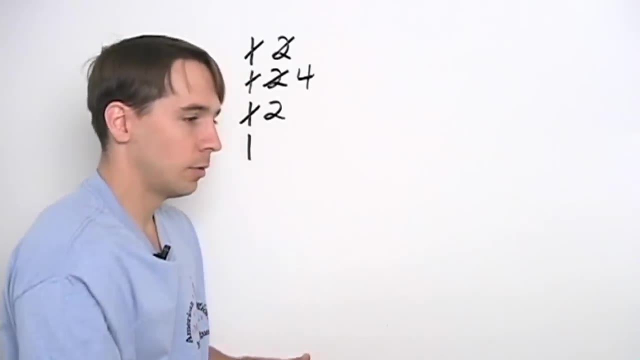 Oh, didn't cheer loud enough, Bet you didn't cheer at all. USA Math Olympiad side. You're stuck at 2.. One more game, One more game. Richard side. You got the Richard side on the first flip again. 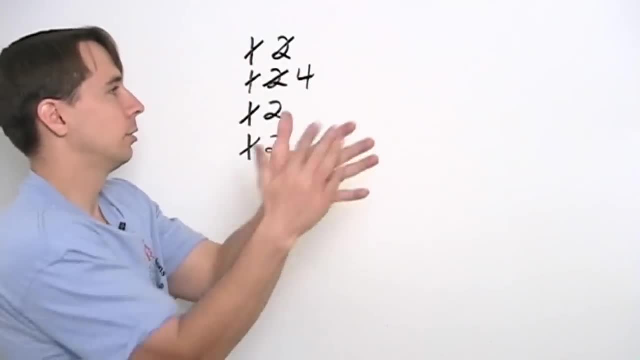 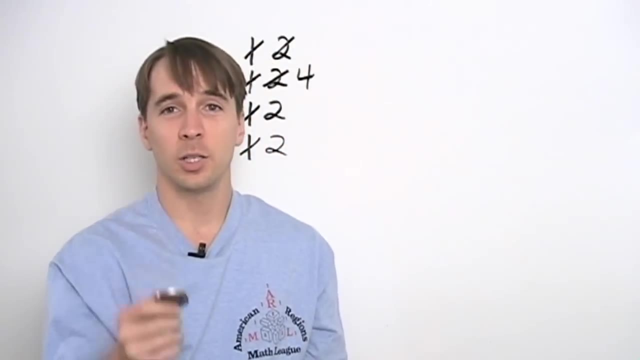 You're very lucky, But not that lucky. You got the USA Math Olympiad. We stop at 2.. So you understand the game now. Here's the question And here's the catch. I'm not going to let you pay for free. I'm a nice guy, I'm not a great guy. 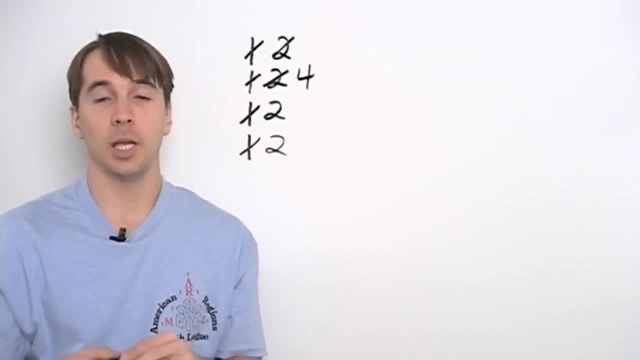 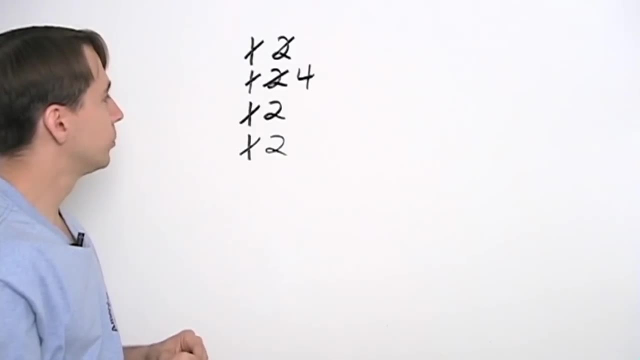 I'm a nice guy, I'm not going to let you play for free. You've got to pay to play this game. How much would you pay? How much would you pay to play? Well, let's see How much would you pay to play one time. 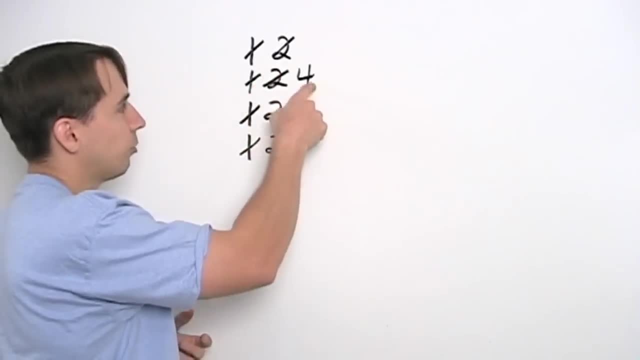 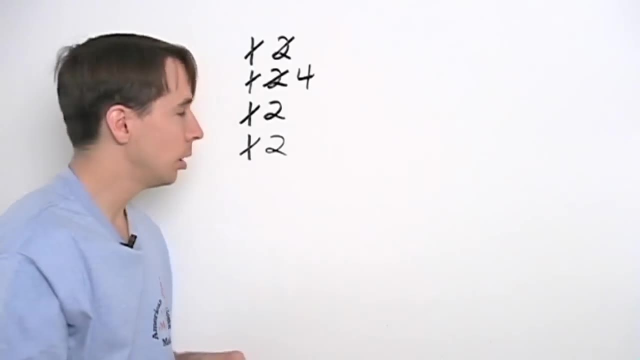 Well, it looks like each time we played. well, we had 4. this time, then 2, then 2.. It doesn't seem like you're going to make a whole lot of money. I mean, you always make at least 1.. So you're going to pay at least 1.. 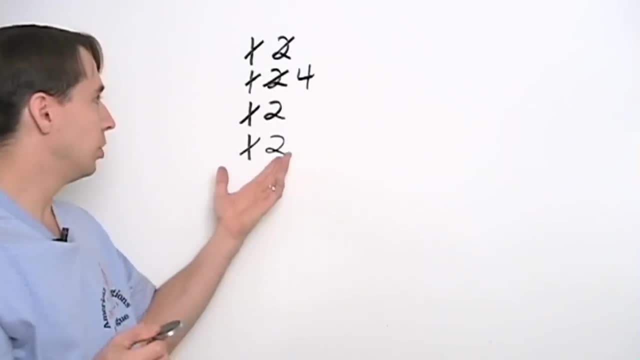 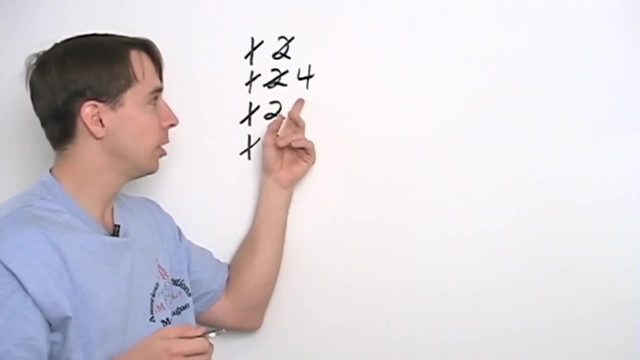 Hmm, But how much will you pay? Would you pay 5?? You never made more than 4 here, But you know, if you'd flipped Richard one more time here, if you'd cheered loud enough, we would have doubled that up to 8.. 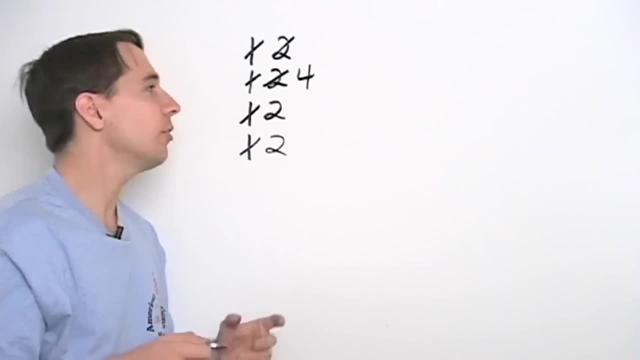 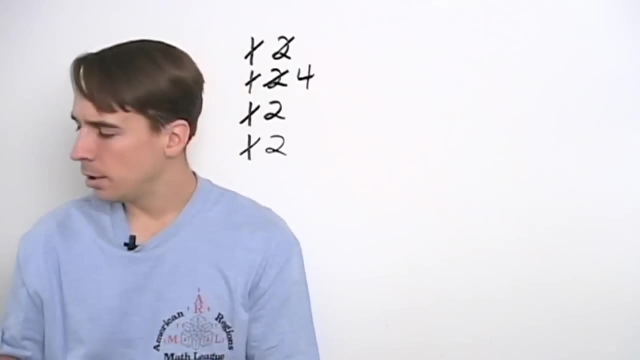 And one more time, we would have doubled it to 16.. So you definitely can make more than 5.. So maybe you do want to pay 5.. What do you want to pay? Let's take a look. I'm going to put my medal down. We're going to take a look at this. 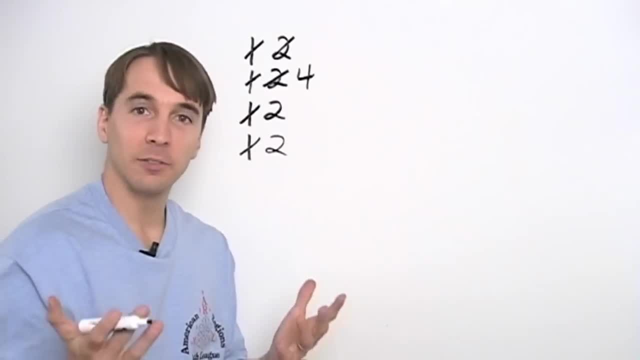 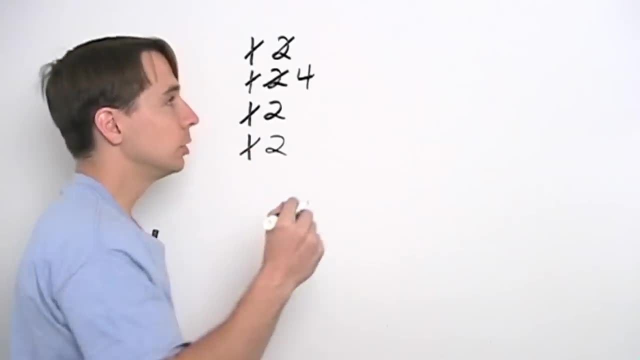 And let's see what happens in this game And we'll compute the expected value to figure out how much you should be willing to pay me to play this game Now. we start with 1.. We start with 1. And I'm going to write that down here. 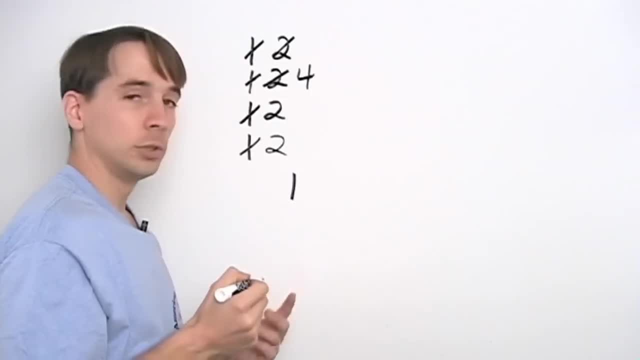 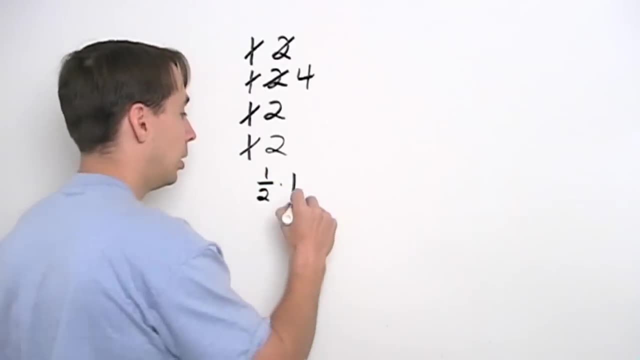 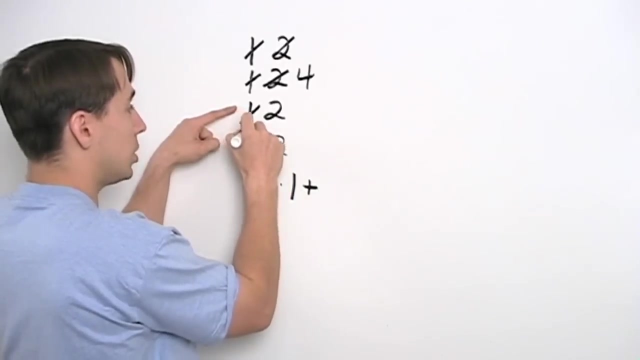 And half the time, that's all you get. You flip the USA Math Olympiad on the very first go And the game's over Now the other thing that could happen is you could flip Richard like we did up here: Richard and then the US AMO. 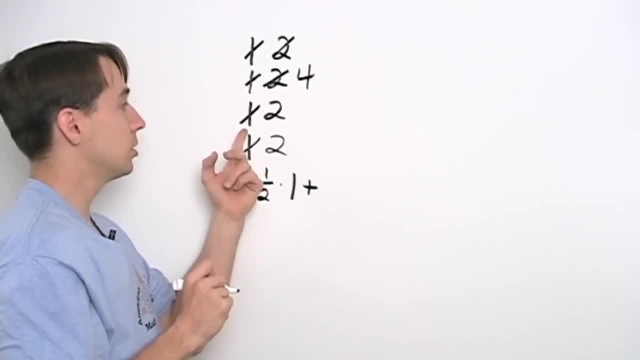 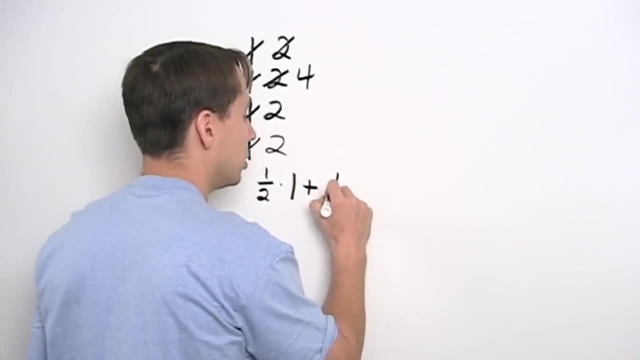 And then you get $2.. Now the probability that happens is: well, you get Richard, with probability of half, and you get the US AMO with probability of half, But you end up with $2 is 1 quarter, Because the flips have to go: Richard and then US AMO. 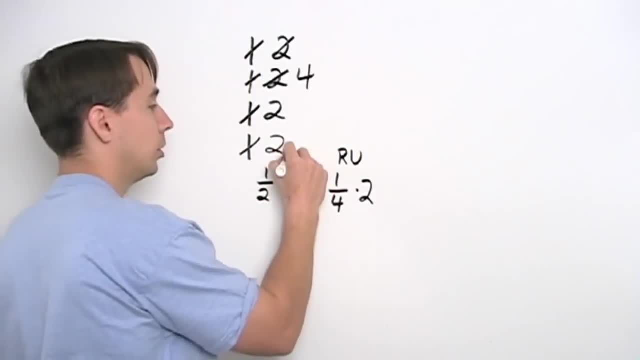 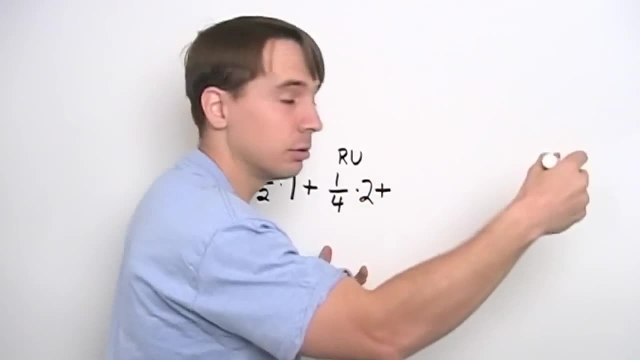 And that's. we'll just go ahead and put that right up there, Put the? U right up here. You get the US AMO. first Here's Richard and then US AMO- Next thing that could happen. you get Richard and then Richard and then 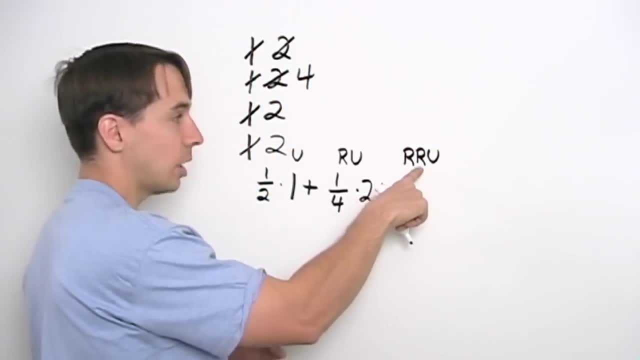 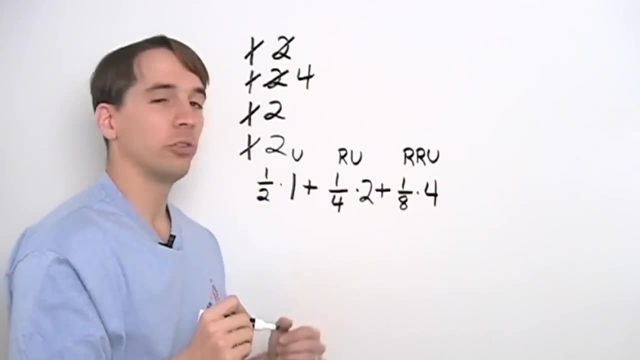 the US AMO, RRU. And that's half times half times half, That's 1 eighth And when that happens you'll get $4 because you doubled twice. See where we're going. How much are you going to pay me? 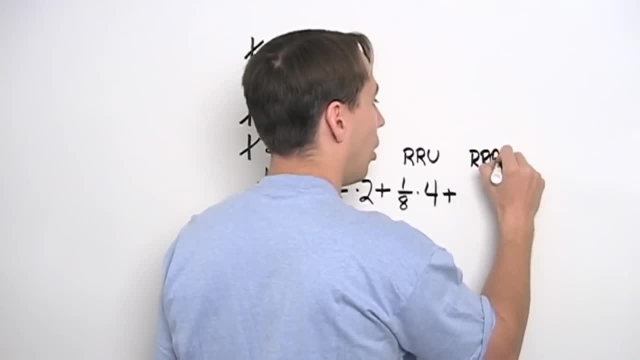 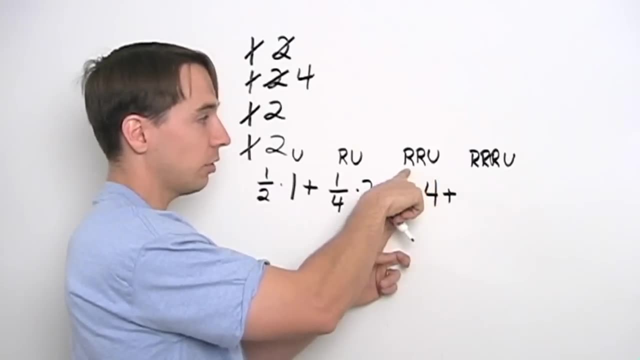 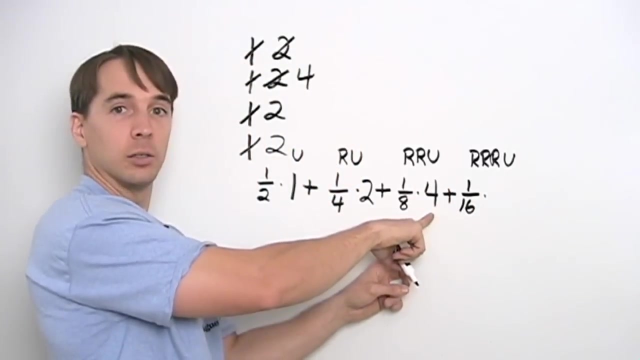 Let's see, You could also get RRRU, And the probability that this happens is half the probability that this happens, Because here we've got the three flips, Here you've got four, But the amount of money you'll make if this happens is double the amount of money. 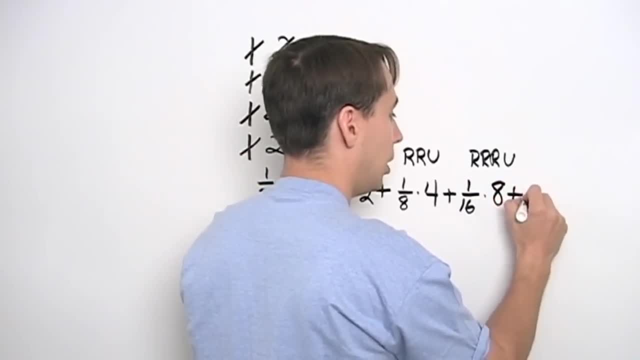 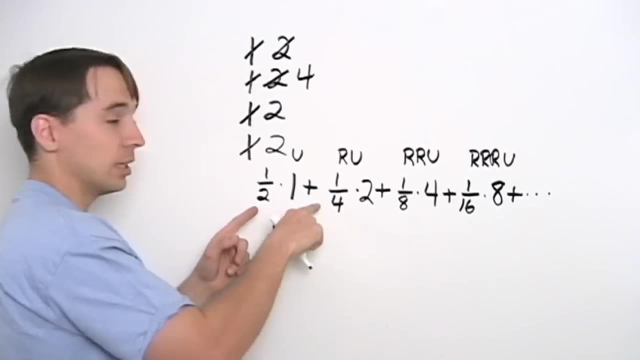 you make here, And we'll keep going like this. Now let's, if we compute these 1 half times, 1 is just 1 half, And then to get to the next step, you saw what we did here. We added a coin flip, So we had to. 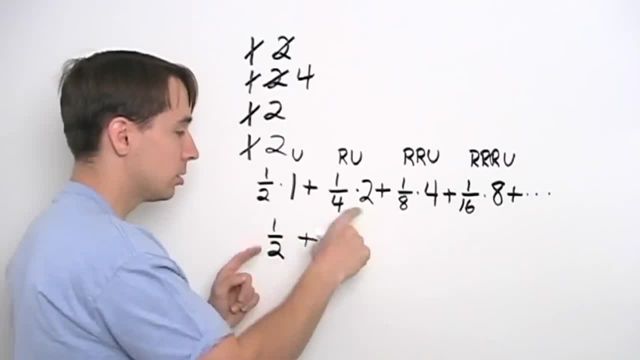 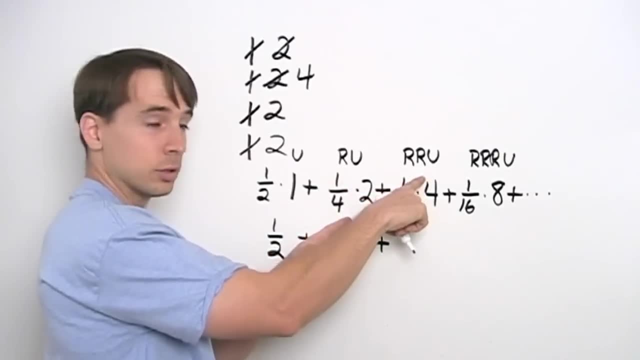 halve the probability that you doubled the amount of money you make. So this product is still 1: half. And then again, going from here to here, instead of 2 flips we have 3. So the probability is halved.